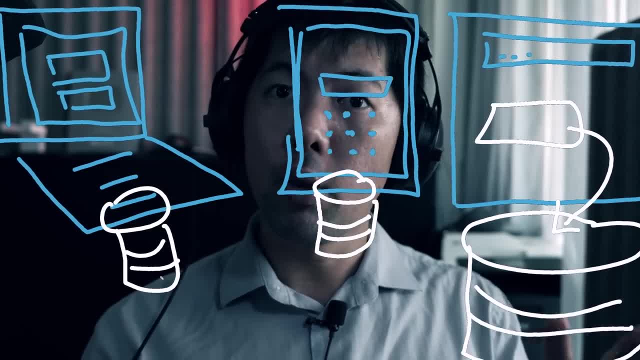 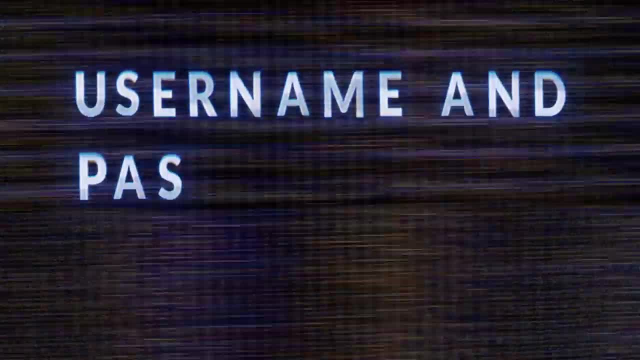 All these different passwords and credentials that you have in order to do the cross-check, And if you get the password right, then you'll be issued, say, for example, a cookie, And, of course, if you get the password wrong, then you do not get access into the site or into the computer. 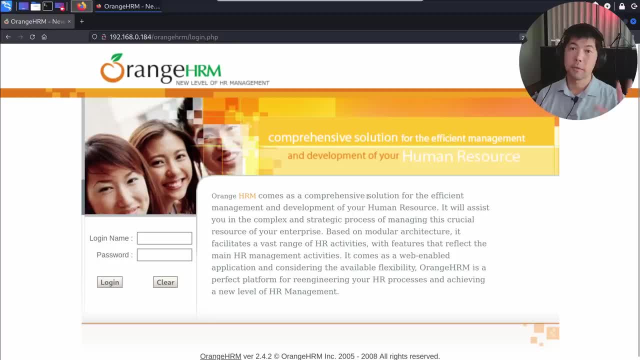 And, of course, our job here today is to learn how to hack it, And right in front of us we're in Collin Linux, which is going to be an article hacking operating system, so that's super cool, And of course we have a browser that's opened up to a website. 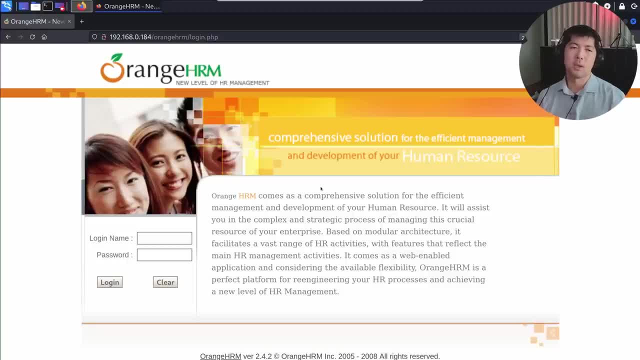 and in this case we can see Orange HRM. So this is a human resource management website And right in front of it we have the login name as well as the password field And typically, if you are a script kitty, you will be thinking about: okay, perhaps we can just 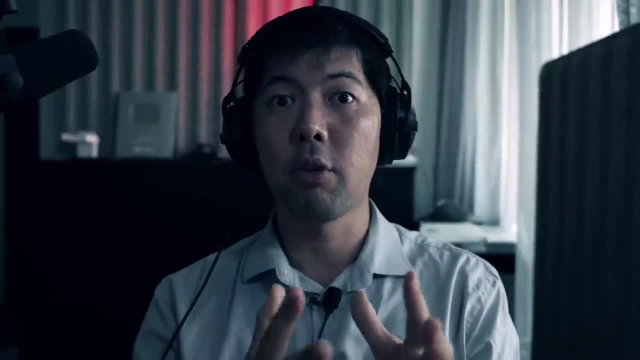 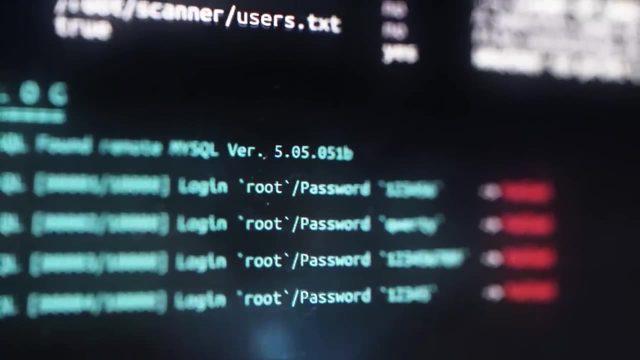 start brute forcing against the site, And brute force attack means we're trying all possible combination of usernames, passwords, possibly those that are much more common, So for example, like admin, administrator, user and so on and so forth- Against commonly used passwords. 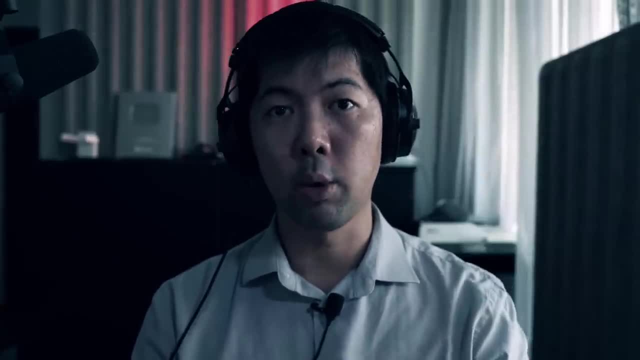 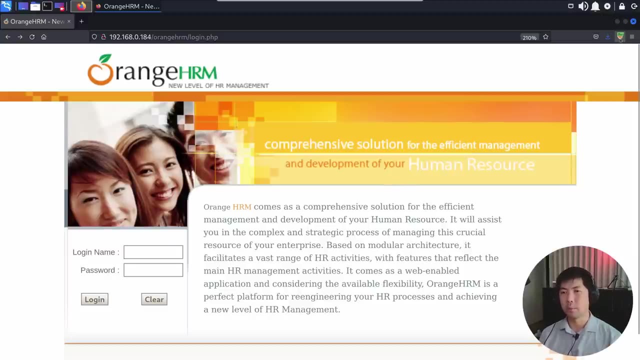 say, for example, like 13345678, password as password, or MrHackerLloyd is very handsome as a password. So, going back to Collin, Linux under the Firefox browser, whichever browser you want to use- you go to the top right corner. 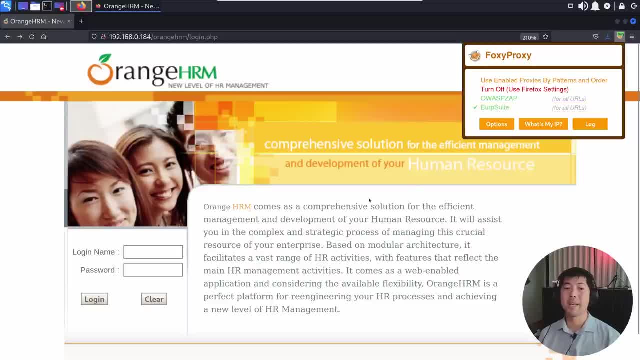 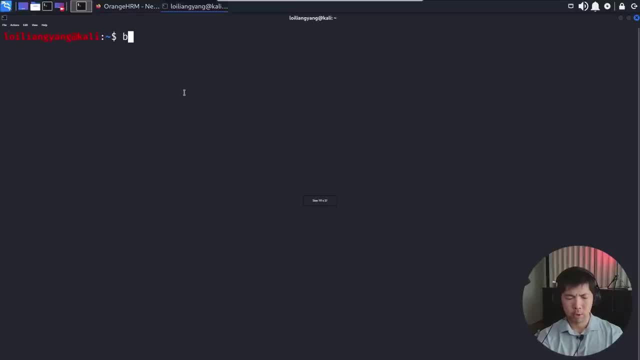 and in this case we have selected BurpSuite on the Foxy proxy, so we'll be intercepting the request. I go over in the terminal which allow us to look super cool like a hacker or like MrHackerLloyd. You have the BurpSuite end, so this will start up our interceptor. 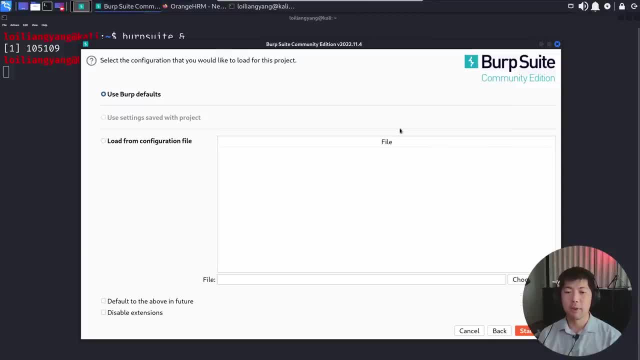 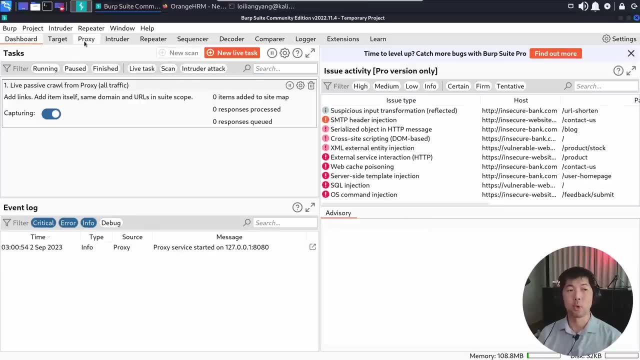 All right, so this allows us to change up the request, modify the request so they're ready to attack the site. All right, so in this case we're showcasing to you what is called brute force attack. So you go to the proxy tab and you see the interceptor. 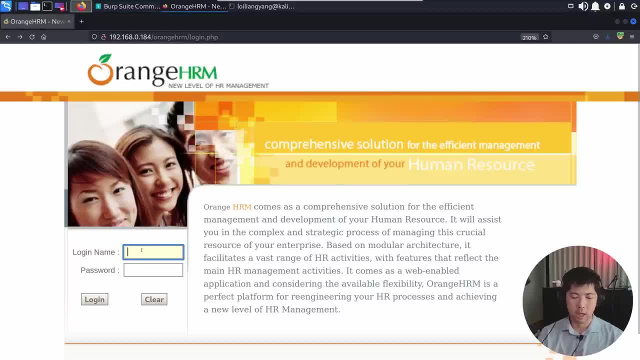 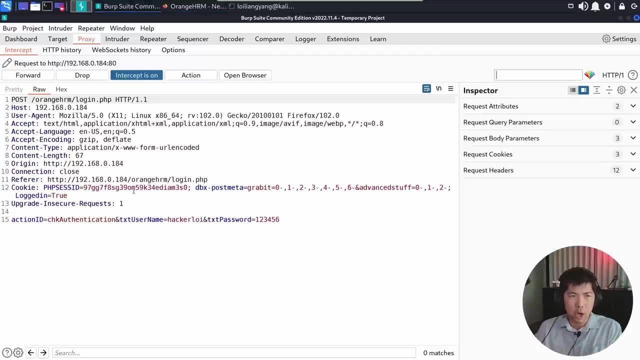 is on. I go back over into the browser, I go and enter, say, a login name like HackerLloyd, and I enter a password. whatever password it is, I don't know the password, so I'm trying it out now. Click login. Now, right here we have interception. I can do a right click. 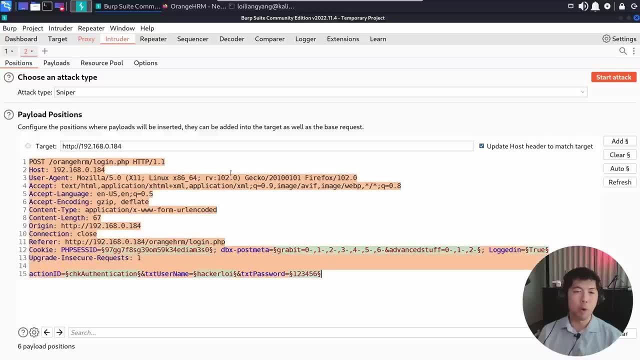 send over, say, intruder and from intruder, I remove all of this, which are our payload marker. So I clear them right here and you can see right at the bottom in the body of the request we have something like text password equal 133456.. 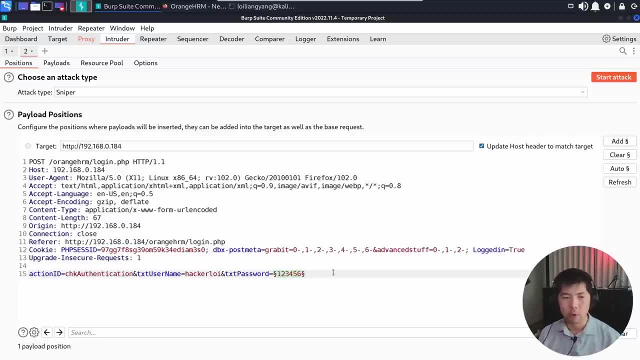 This is going to be the one that we'll be adding as a payload marker, which means that we'll supply a list of payloads that we can change up as the potential password. So I go over the payloads on the second tab and I can load right here under the payload options, Click load and right here. 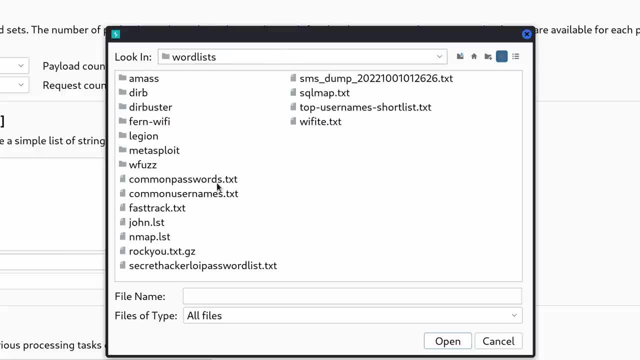 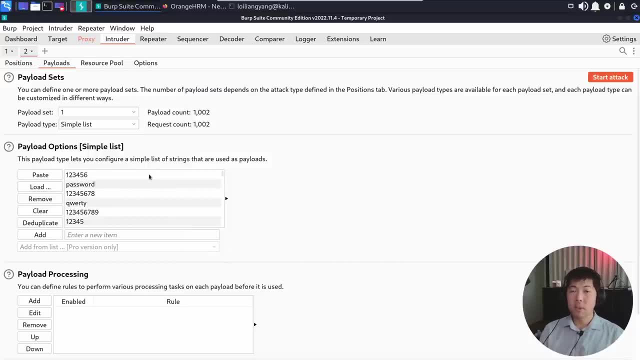 we have, say, for example, word lists and we can possibly use commonpasswordstxt. So let's go ahead and double click on that and we have a list of all the different passwords here. So once you're ready- all right, as simple as that- go to the top right corner. all right click start. 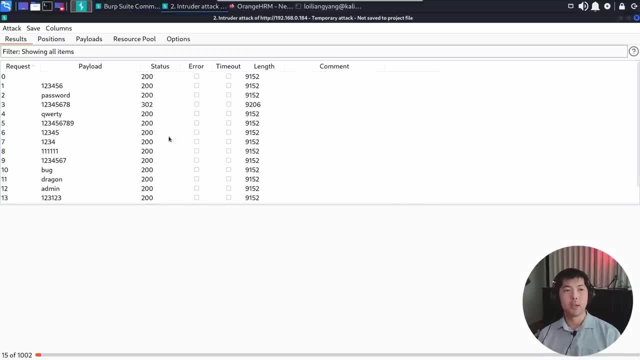 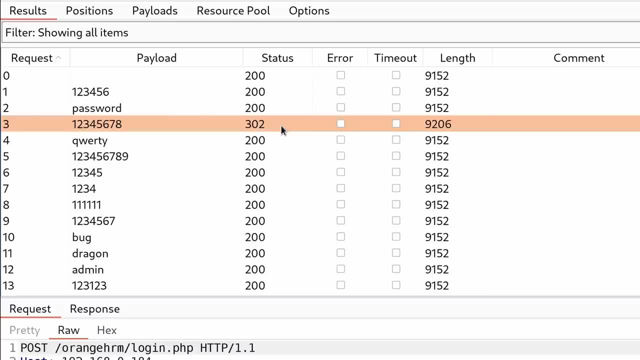 okay, and the attack is going on right now. okay, So once we have that, we see something very interesting. all right, So possibly helping us highlight what are the potential passwords that we can use as part of launching the attack So I can pause the attack right here now and you can. 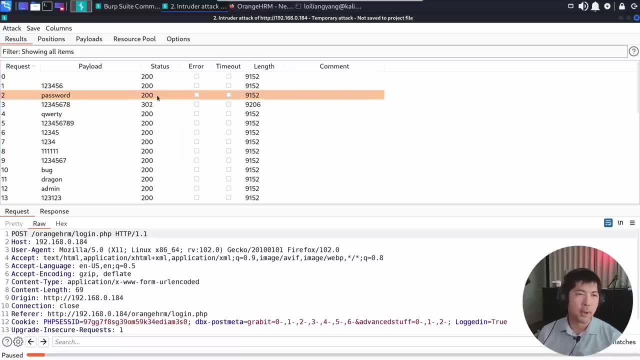 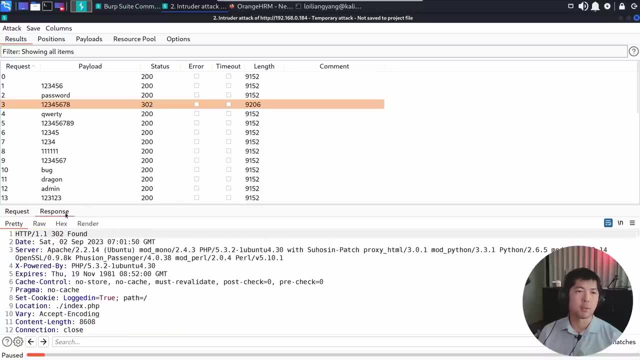 see right here we have the status all right. So we have like 133456, password is password, and so on and so forth, And the one that stands out the most is 13345678.. So from here I can click under response and you can see, over here we have certain information. 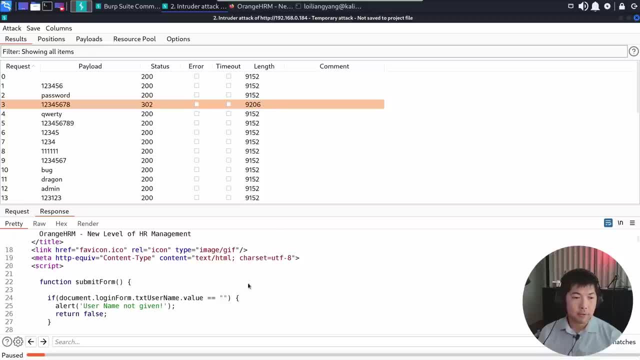 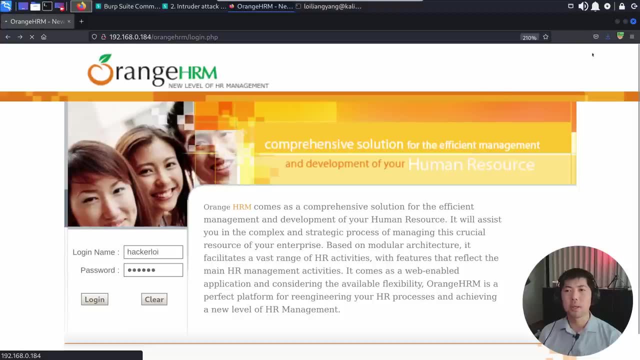 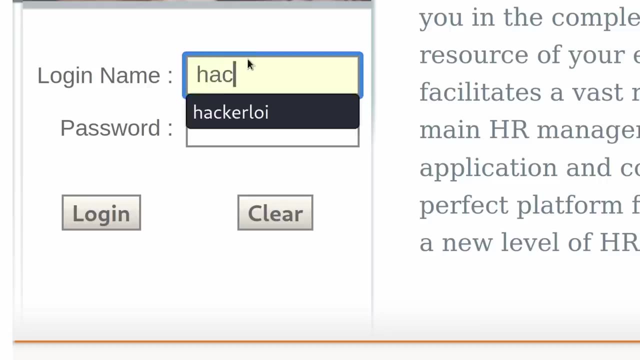 all right. So 302 9206 length. so this is very different from all of the other attempted values. So if I go back over to the login page, I can go to the top right corner and I can turn off. turn off the interception. right now I go ahead and do a refresh of the page and I enter hacker. 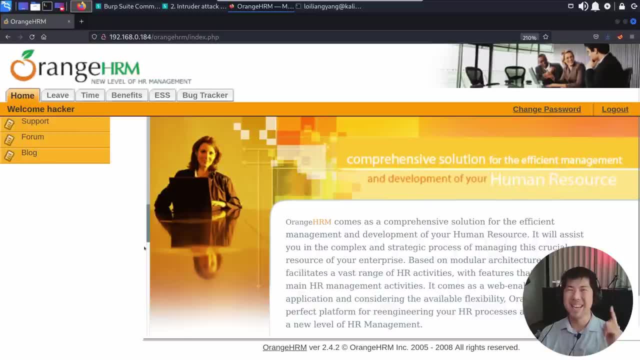 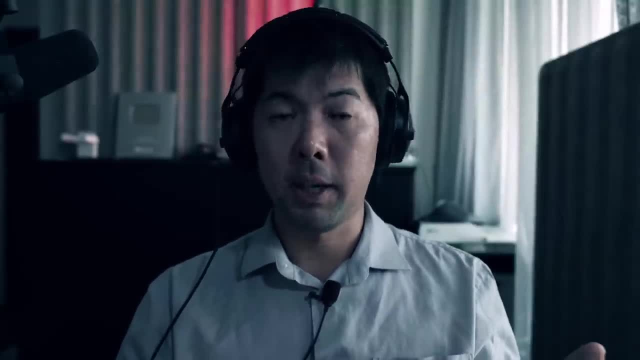 law, followed by password 13345678, click login. boom in done. You've hacked into the system now, And this is the easy part of hacking. but this usually gets blocked out really quickly by some web application firewall on the front end or, at the same time, an application logic where 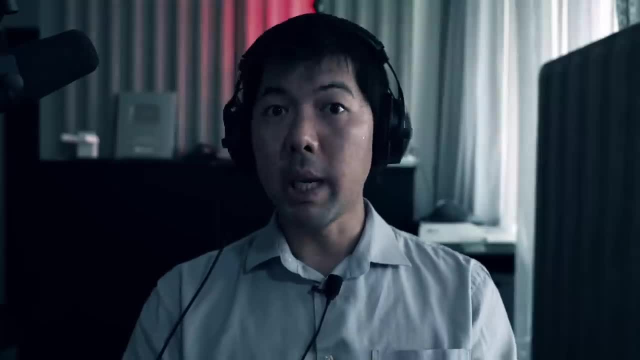 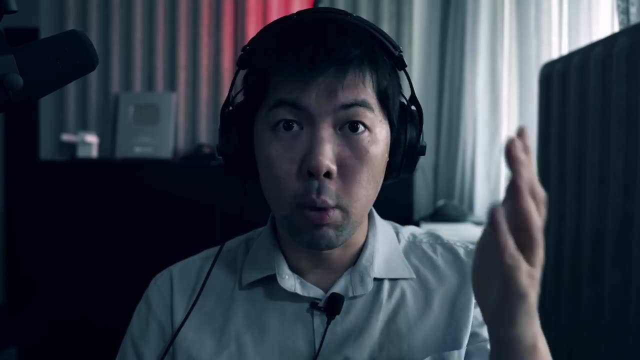 say, for example, you attempt five times, or more than five times of incorrect password, they block you out. So we want to think about something more creative. We are better than doing a performance attack. So you're not script kitty, You want to be as good looking as Mr Hacker Law. 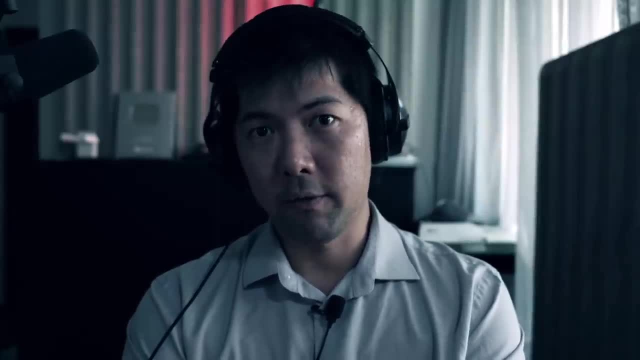 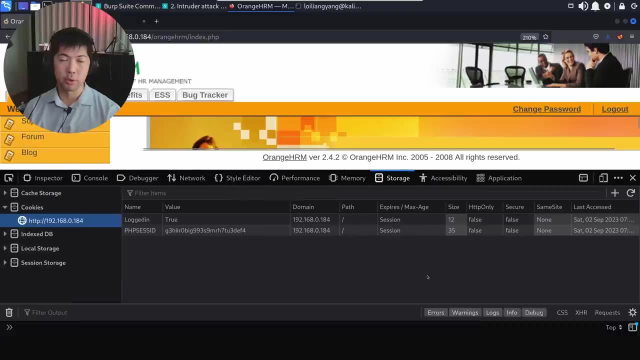 sorry, I mean, or as cool as Mr Hacker Law, then you have to be more innovative than that. So, going back to the target website, what we can do here right now is go to the top right corner, click on our raw tools, web developer tools and on the 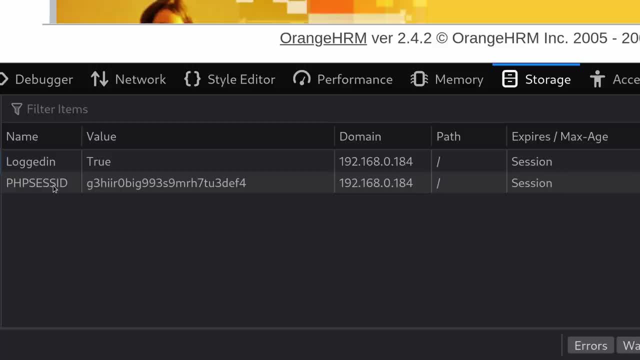 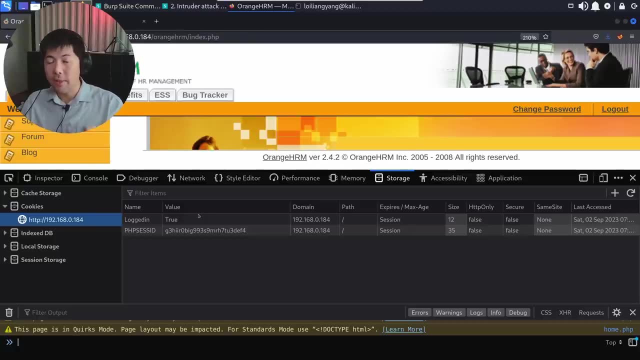 storage. what we have here is PHP session ID logged in, and we'll be using these two values to help us copy these cookies, which means that we're going through an authenticated session so that we are able to use those scripts and tools to crawl through the site, looking out for potentially 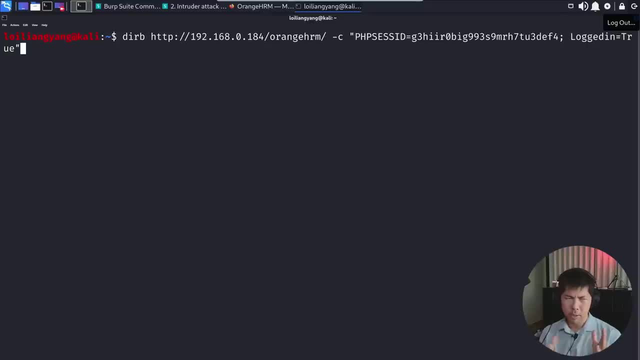 different types of pages, directories that we can go after. So, going back to Clonolix, right in front of us we have DRB, which is for us to crawl through the site looking out for different pages, directories of interest that we can target, And, once you're ready, go ahead. 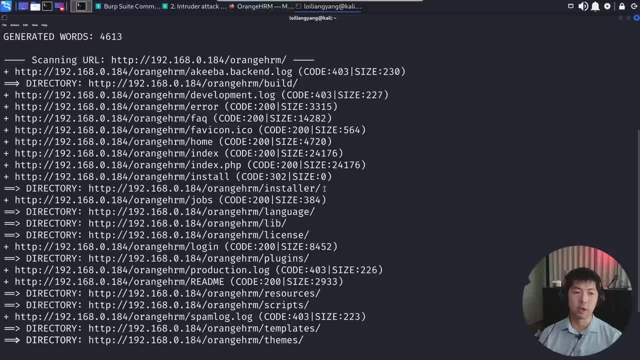 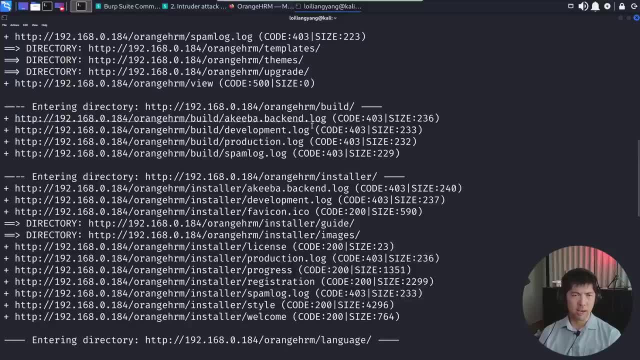 and hit enter. and now we're crawling through the site And you can see right here: look, we got all those interesting things, Installer. all right, we have the build, we have teams upgrade templates. So we're crawling through further down into different 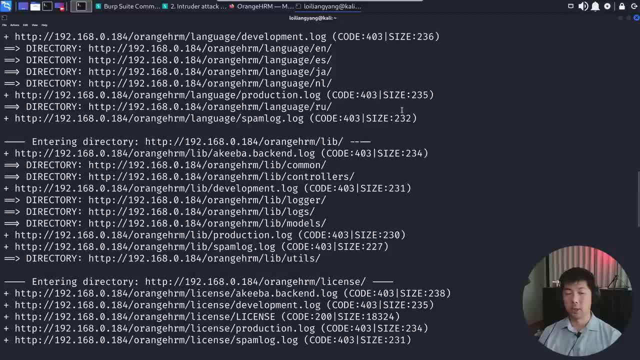 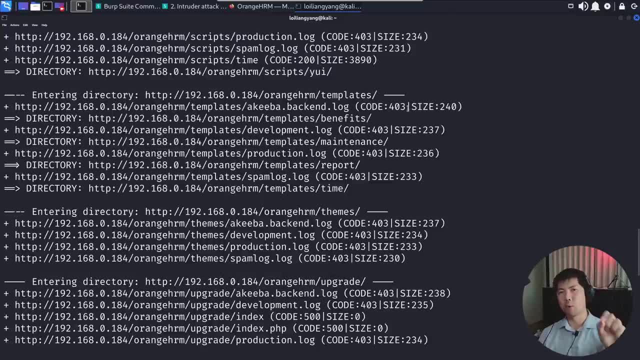 parts of the site where we can find things that are very interesting. Okay, So at the same time, let's go ahead and let the script run So we highlight those things that are most important for us to possibly discover vulnerabilities with the site that can then give us. 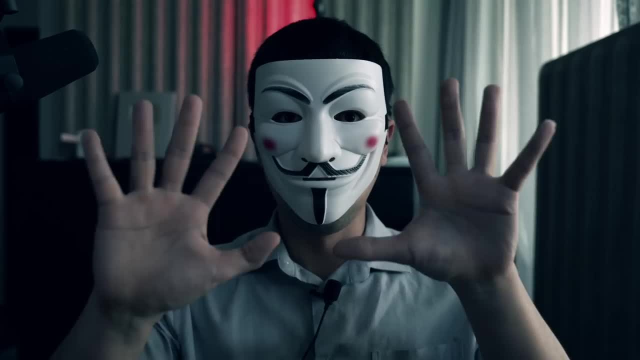 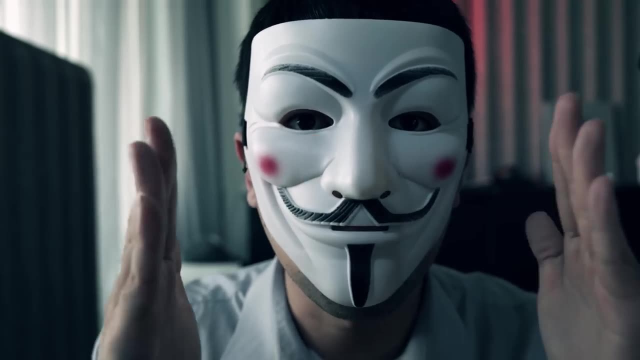 access to the backend database system. Now remember kids, before we continue further. hacking is illegal. The only reason why you want to learn hacking is because it's so they can look as cool as Mr Hackaloy. Now look right here. the scan has completed. We're able to uncover: 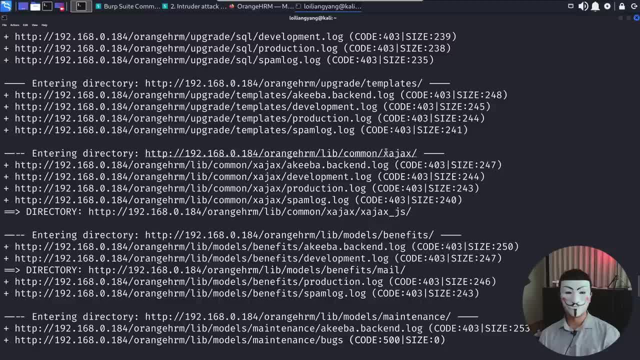 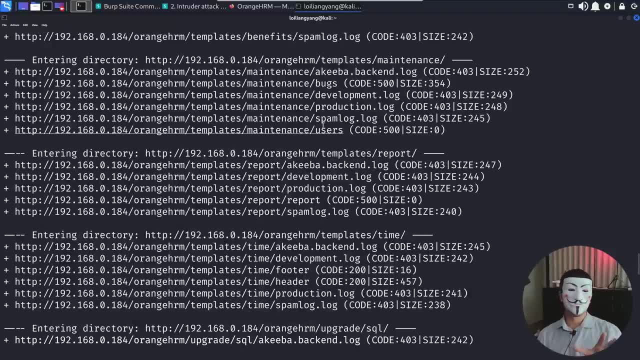 lots of different directories And we have say, for example, Leap Common, XAJAX, Templates, Benefits, Maintenance, and so on and so forth, So we're able to discover all those different directories as well as possible files or different parts of pages that 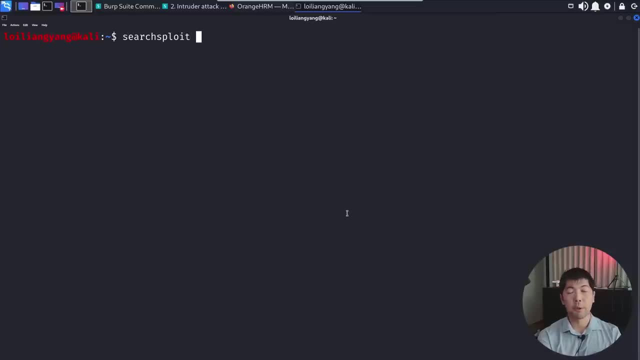 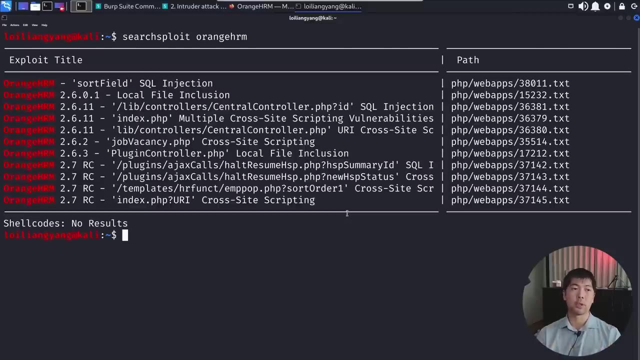 we can target. At the same time you can also use SearchSploit to look up for potential vulnerabilities and weaknesses in relation to, say, RNGHRM. So if I hit enter on that, you can see right here we have the following information. So we have, say, for example, SQL injection for salt field. 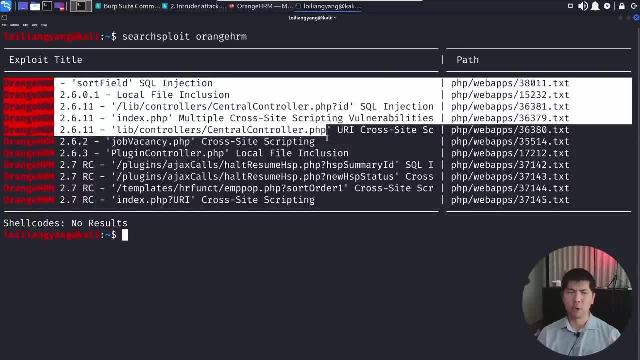 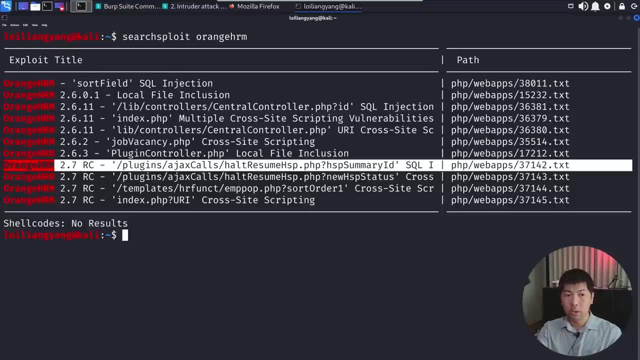 local file inclusion, central controller, multiple cross-scripting vulnerabilities and so on, So you can easily study them up. So in this case we can target, say, plugins, AJAX calls hot resume, HSP and so on and so forth. So possibly this is something we can. 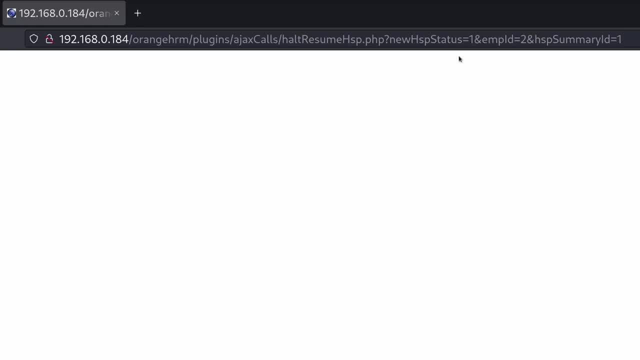 do So. I've opened up the browser one more time And what I've done here is I went ahead and entered into this specific link or this specific directory with this PHP file And I entered following a new: HSP status equal one, employee ID equal two. HSP summary ID: equal one. So it states that this is. 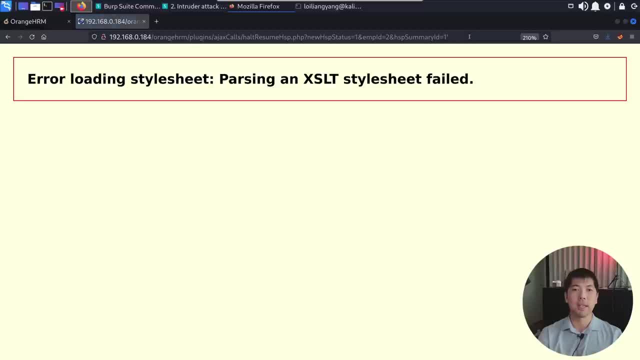 susceptible to structured query language injection. If I put a single code here and enter that, it gives me some kind of error message indicating that possibly, yes, there could be some kind of lack or poor sanitization behind the scenes. So we can target this Next up. 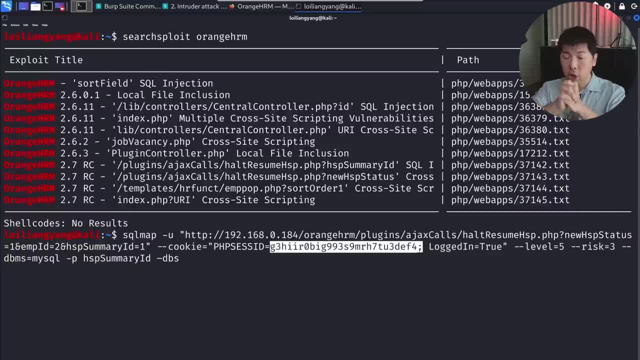 because we understand that it is a structured query language injection vulnerability. we can use SQL map to help us with our SQL map. however, we want to call it So right here you can see we're targeting RH, HRM plugins, AJAX calls and so on and so forth. 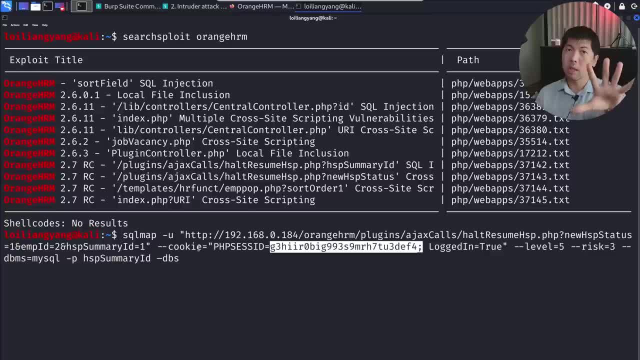 summary ID, equal one, And we have the following of cookie. So this is the cookie value that we have from the start of the session And we log in equal. true, We have level risks As well as the DBMS. So in this case, when you're searching and understanding about a specific 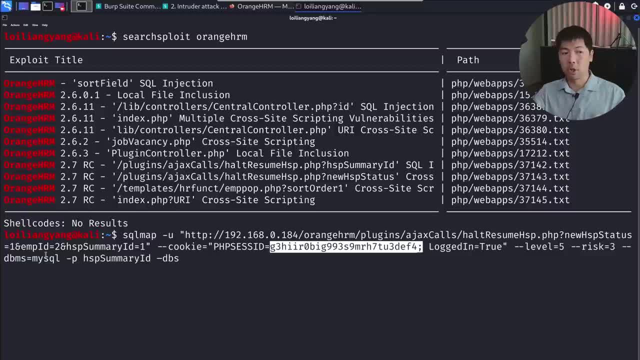 whether it's content management system or a human resource management system like RH, HRM, whatever it is, you want to understand the structure behind it, And the good thing is a lot of all this open source type of systems. their code is out there, So the structure is. 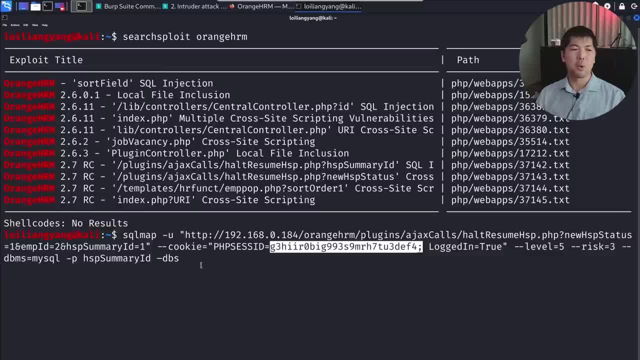 out there and you can easily try to understand what's going on. So in this case, we are also targeting HSP summary ID and then followed by DBS. So what we're trying to do now is to think about what is the databases that are available, What are the databases that are available? 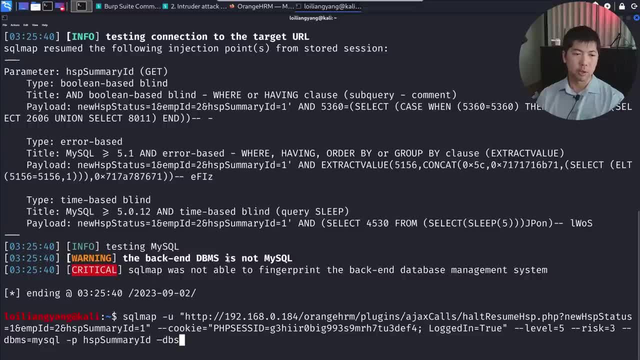 What are available for us to target. So go ahead and hit enter on that. And, of course, so let me just go ahead and put a double dash on DBS and we can see the following results. So perhaps sometimes you don't want to indicate, say, DBMS, All right, so let me remove this one. 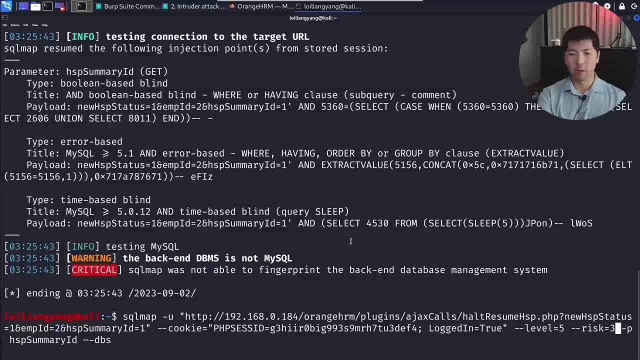 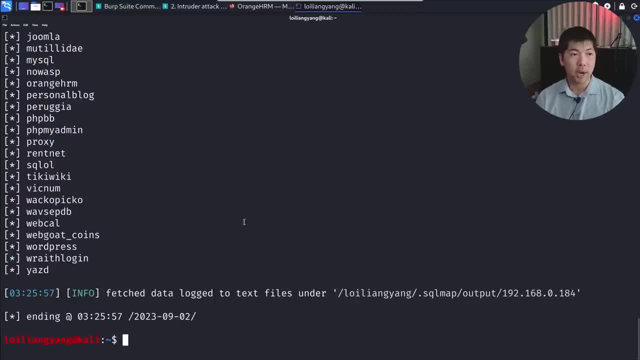 and let me just go ahead and remove this too. Go ahead and hit enter on that and boom done, And we managed to dump out all this different information right here. You can see the following: So we have, say, RH, HRM. We have possibly other different databases within. 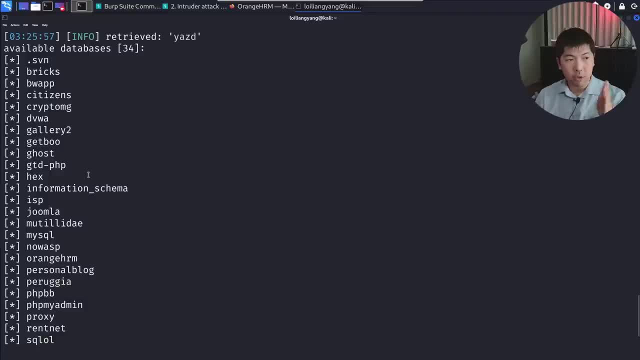 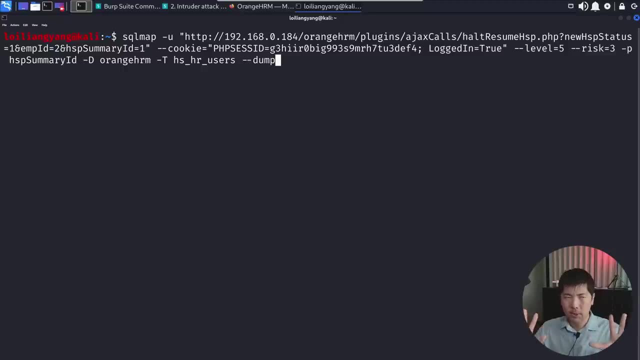 the backend. So these are all the databases that we can target. So, of course, in this case, we're going after the orange HRM database Now, because we started the backend system. So what we can see right here is we're using SQL Map, targeting the same entry point once more. 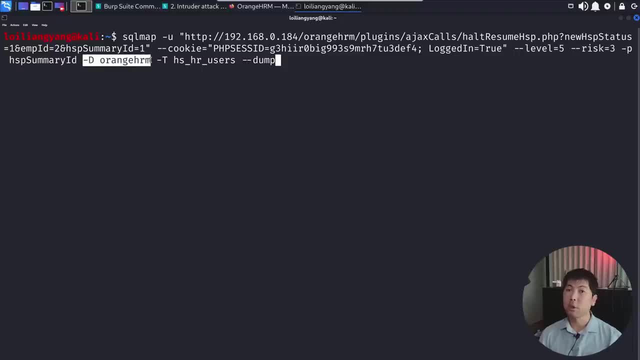 but now we are highlighting here dash D for target database, dash T for the table. So within the database there are many tables or possibly even one table. whatever the case is, We have HS, HR, users, dash, dash, dump. So we're targeting the database. Now we're targeting the table. So 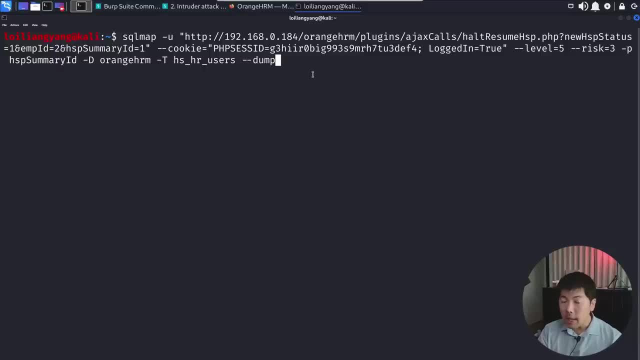 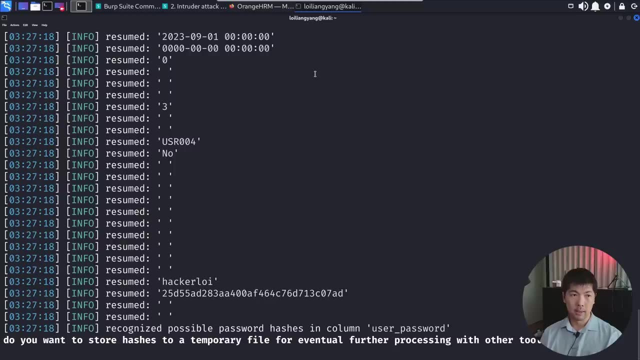 we're trying to dump out all those information within HS HR users which can possibly contain the password field tool. So let's go ahead and hit enter in. three, two, one boom. You can see right here we've got the following information: HackerLoy, as well as some form of possibly. 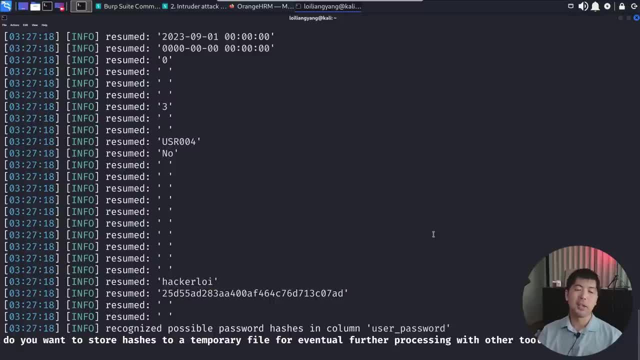 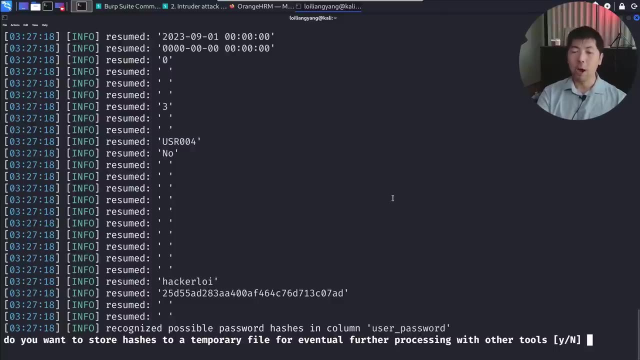 protected password. And the good thing is out of the box. SQL Map allow us to store this into a file In this case. I want to highlight here that I don't really want to store this for further processing in the future. I want to attack it right now. So what I can do now is go ahead and 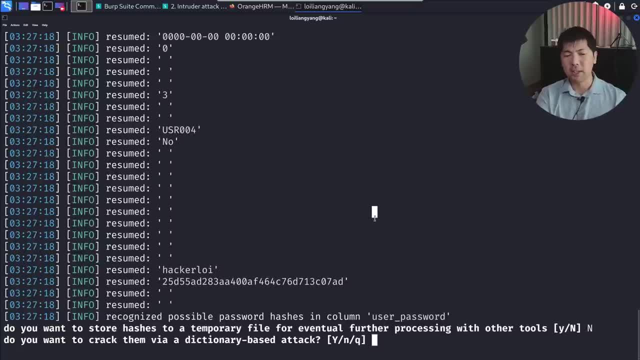 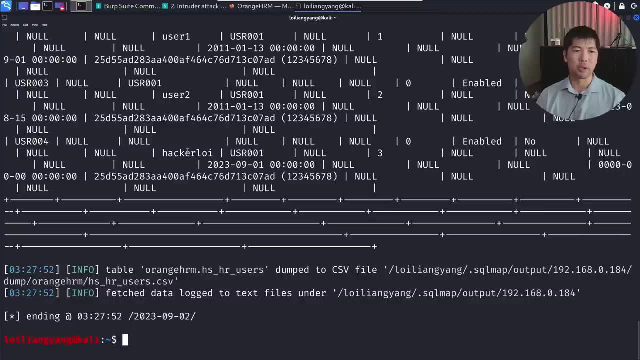 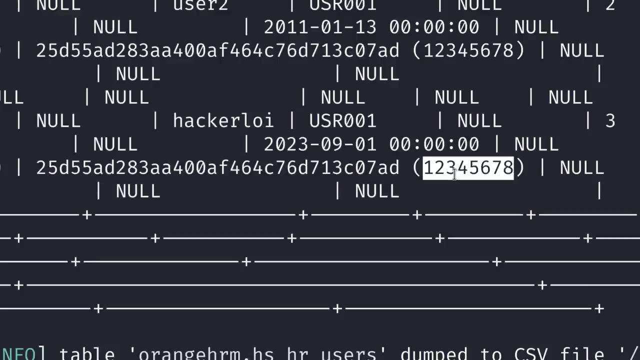 enter: no. Do you want to crack them via a dictionary based attack? Yes, Boom Done, All right. So if I screw up a little more, we can see right here we have HackerLoy, We have the protected password, All right. So again, this went through some kind of hashing algorithm And now this is. 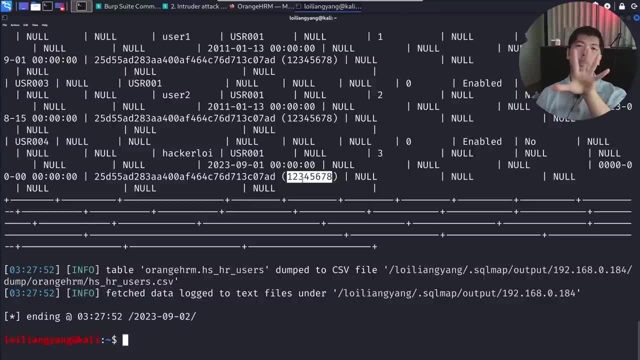 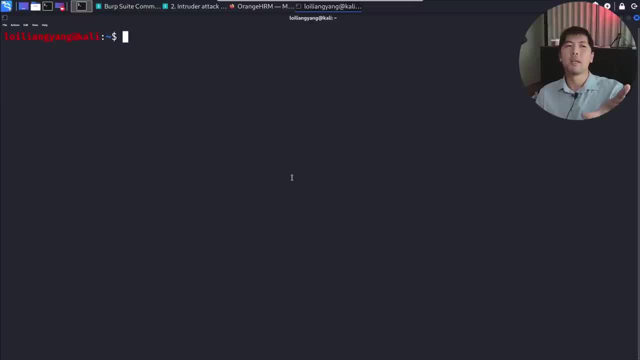 a password of 12345678.. So we managed to attack the password. but it's not all the time that you manage to crack those passwords, because the first thing you need to know is to understand what kind of hashing algorithm are they using. So what you can do here is enter. say, for example, you have 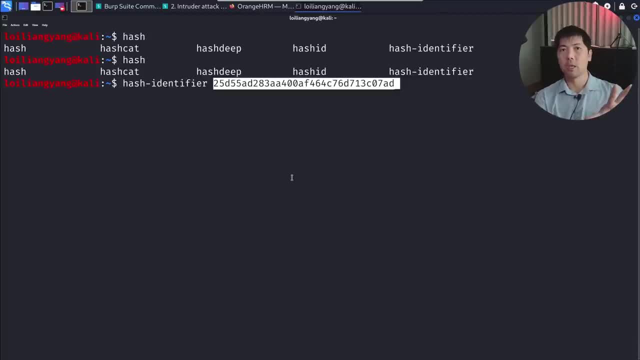 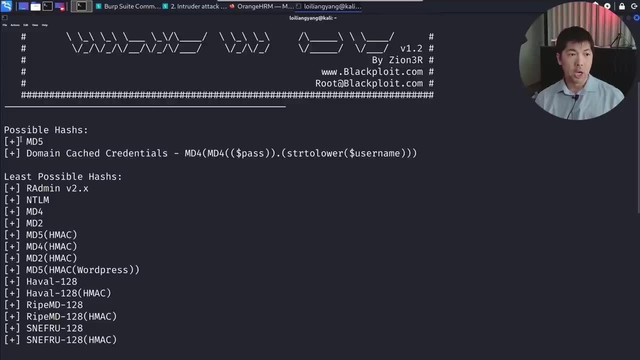 the hash identifier and it can paste the value right here of whatever information they've gotten from the backend. You can enter on that and it can see right here. It tells you that this is based on a possible hashes of, say, MD5.. So what you can do now is you can go over. 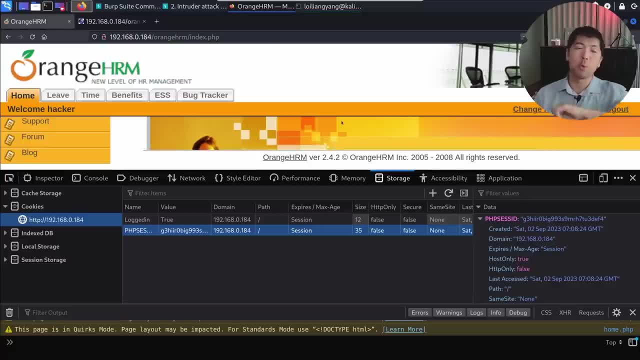 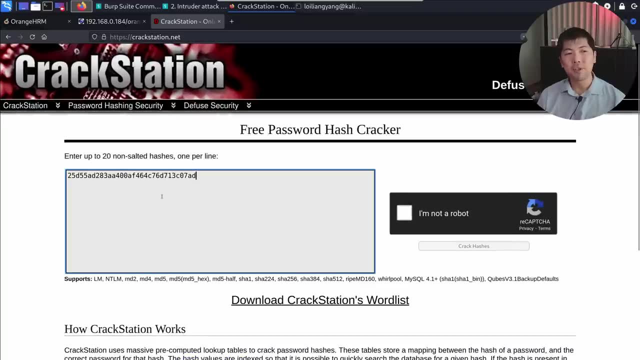 into something called the rainbow table that we can use to do a reverse lookup and see whether we have those unique value available there. So right here I'm on a website called crackstationnet. I paste the value right here, I select, I'm not a robot, I click crack hashes And you can see right. 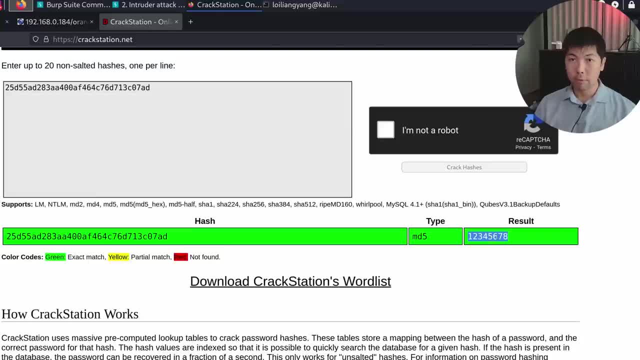 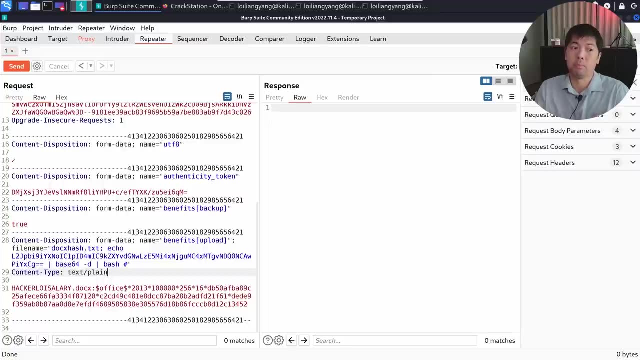 here we have following results: All right, We have a result of 12345678 as a password and a hash value on the left. So this helps us speed things up just by throwing hashes into the web site, which then allow us to look at all this possible already saved value In other situation. 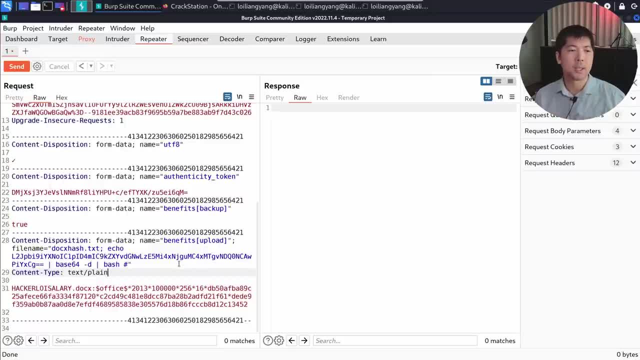 you perhaps found another vulnerability. So in this case you can see on the left side we have an operating system command injection. So perhaps you only got a reverse shell. So if I go ahead and click send and I go back to one of the terminals here, 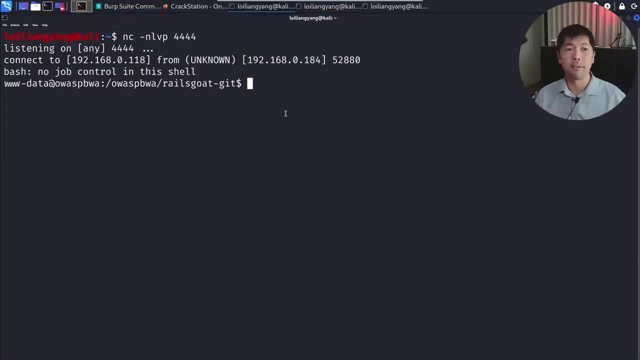 So, for example, in this case I have the terminal here and we have a reverse shell. So perhaps with the reverse shell you now have an access to the operating system And perhaps say, for example, we know where at C shadow is. So if I was going to call cat, 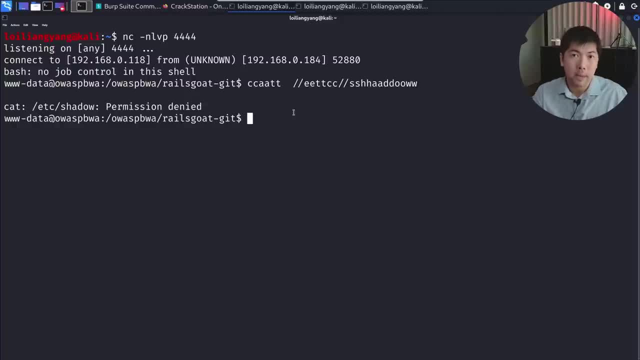 all right at C shadow. I hit enter on that, permission denied. So we're not running with an elevated privilege, So we're not able to view certain important files. However, we may be able to find other locations that hold credentials like usernames and passwords. 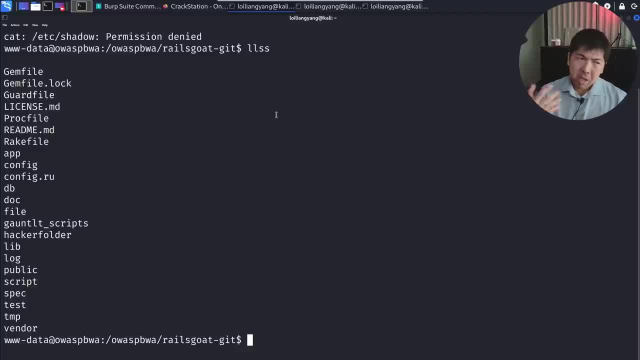 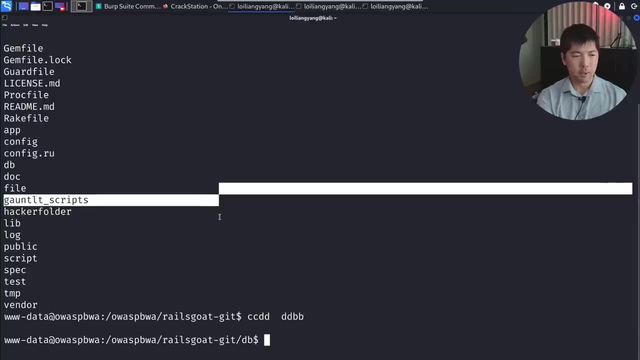 So in this case, if I go ahead and enter, say, for example, LS, I can see the following results, And the one that may be useful for us is DB. So I can go ahead and CD over into DB. All right, I can enter once again, enter LS, And I can see over here. 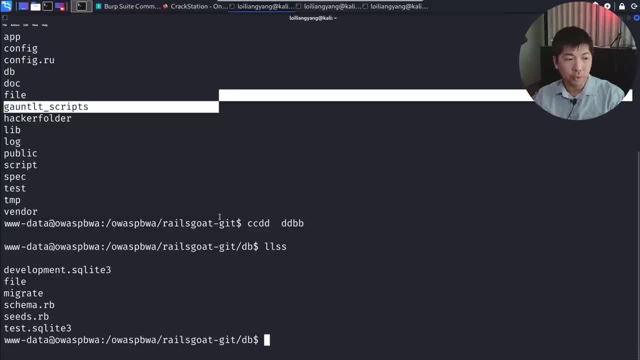 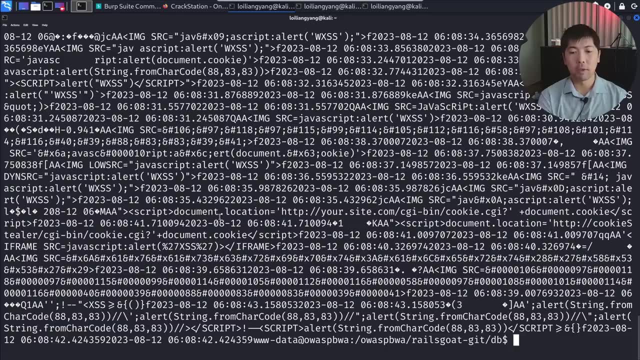 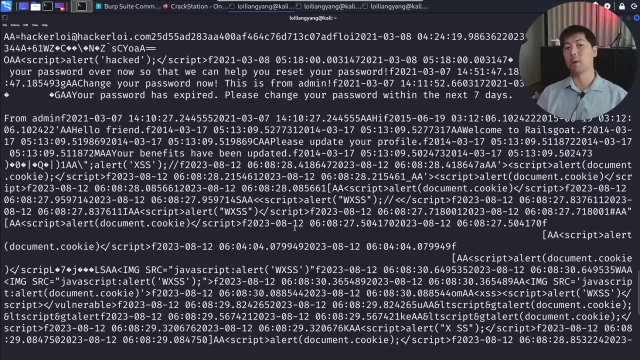 possibly developmentsqlite3 could be a target, All right. So if I go ahead and say I do a cat developmentsqlite3, we get certain results out of it, All right. So possibly it may contain some kind of very useful information that we can use as part of. 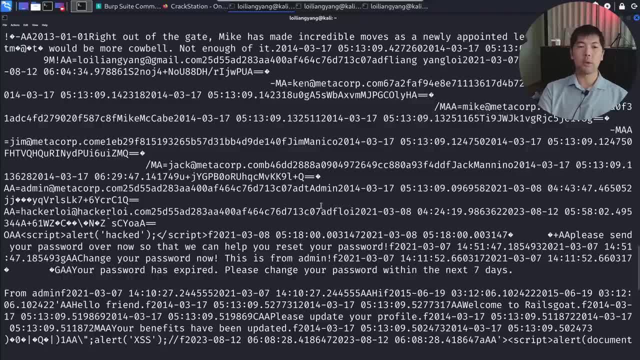 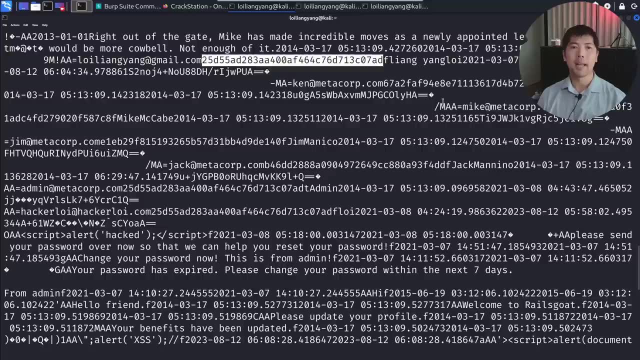 finding out where the password is, And just by looking at this alone, you can see some results that may be containing some kind of important data that we can use. So, for example, over here we have loyliangyang at gmailcom followed by some interesting values. All right, Likewise. 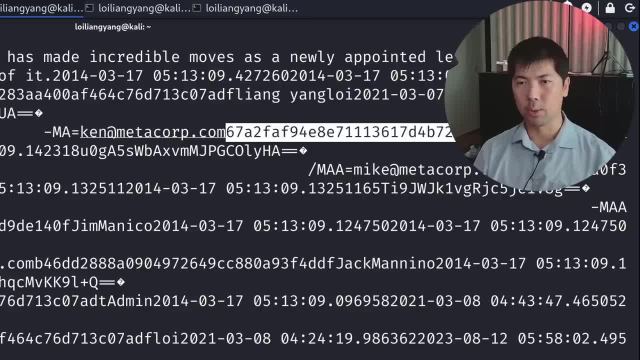 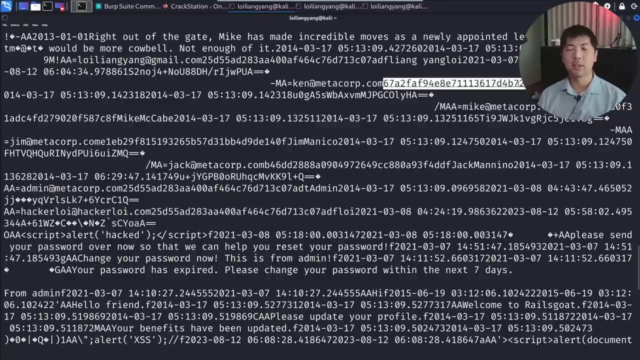 can at metacobcom, followed by some interesting values. So this could possibly be ways where we can gain access to other parts of the operating system that we can use. All right, So let's take a look at some of the things that we can do here. 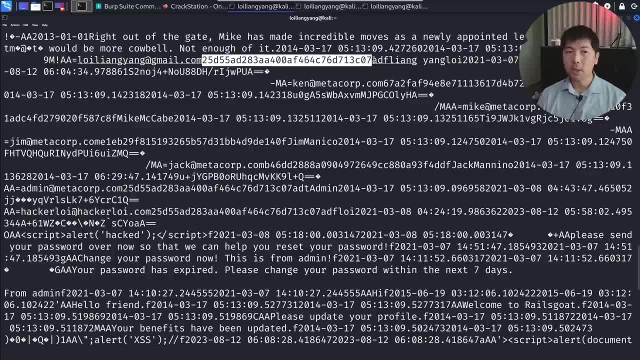 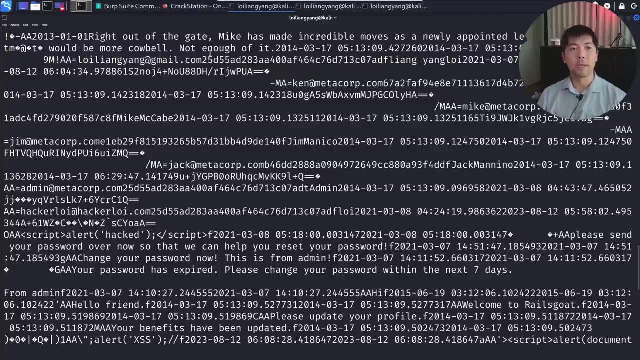 So let's say we're targeting a credential Say, for example, we're targeting Mr Heckerloy, So you can see the value right here. That's right after the email, which means that this could possibly be the subsequent column that contains the password value. So, with that in mind, what I 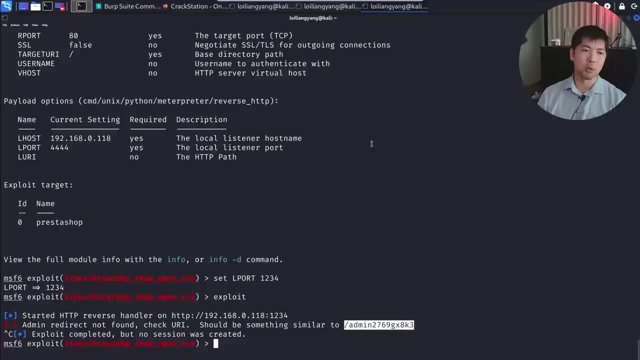 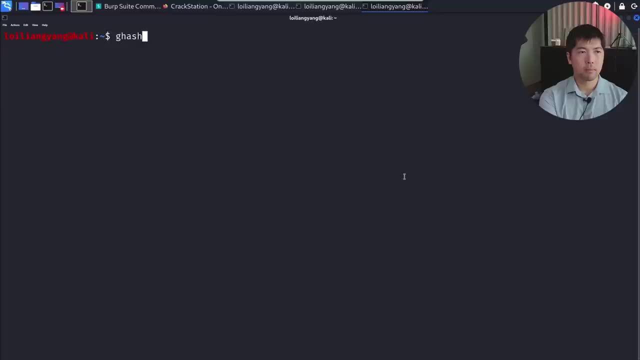 can do here is: I can go ahead and copy the value here. Okay, I do a say copy selection and whatnot, And I can go over into the hash identifier once more, So I can go and exit on this one Identifier, followed by the value. I hit enter on that and it says the following: All right, So we. 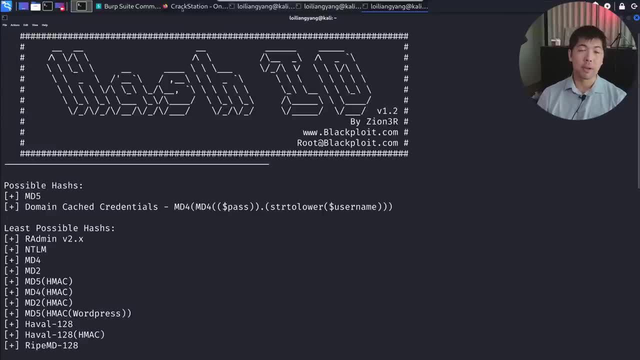 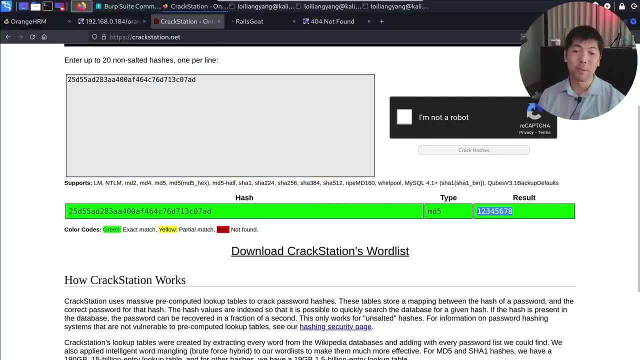 have the possible MD5 hash value. If I go over to crack station, you can see right here we have exact same value And this means that the password is one, two, three, four, five, six, seven, eight. 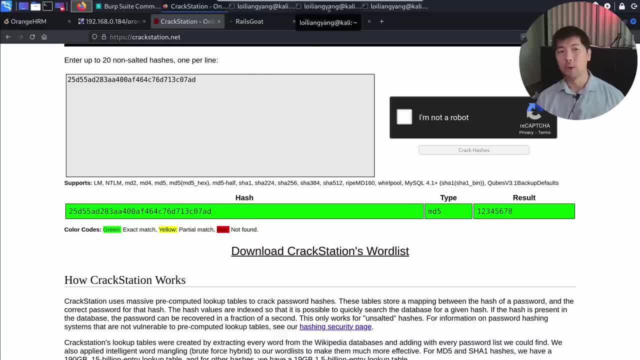 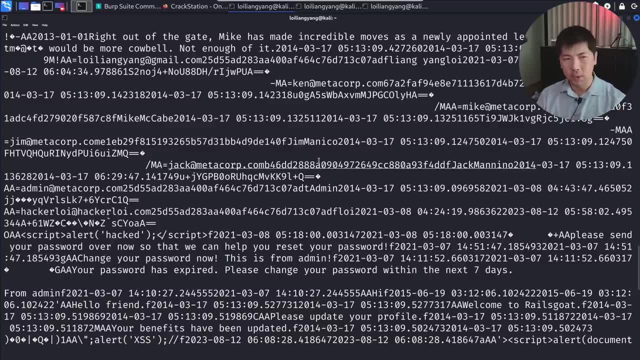 And we also have many other values within the file. So possibly because we have access to the file, So sometimes we may not have access to all of the files, but we may have access to where some of the data might be. So when we look at the hash, especially in, for example, like configuration, 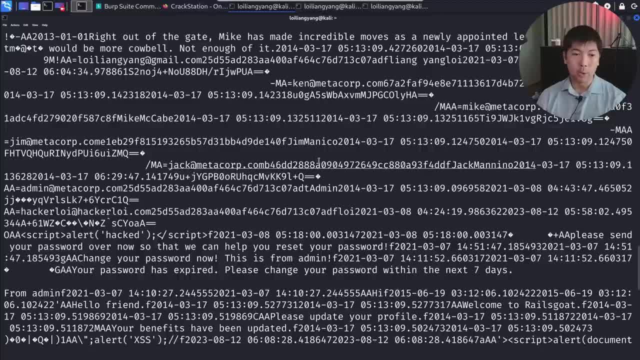 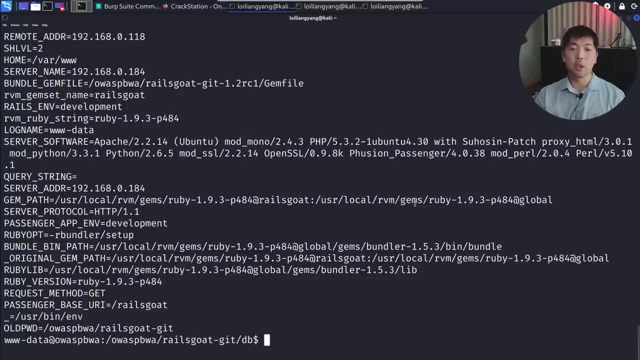 files in environment variables. they may be holding those very useful data that we can use as part of targeting or attacking the password. The other location we can enter: ENV. hit enter and it shows us a lot of interesting information that we could possibly use. So sometimes some of it may.